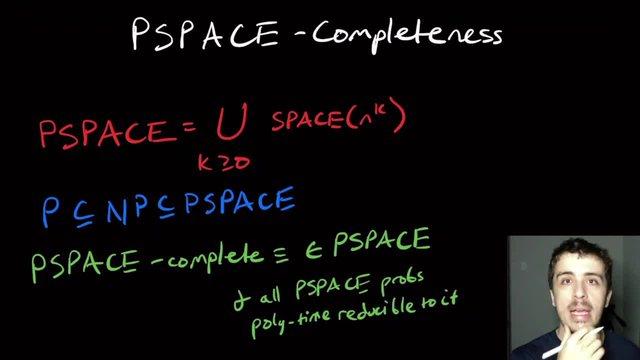 to look at polynomial space, And one thing that we can prove pretty quickly is that p is a subset of np. We've already known that so far, but np is actually a subset of p space. So any problem that can be done in non-deterministic polynomial time can be solved with a polynomial amount of space. 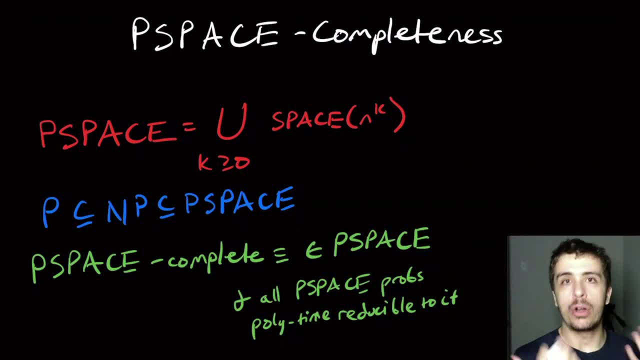 And the way that you prove this is actually very easy. All that you need to do is to find any example of an np-complete problem, like sat, for example, that can be solved in a polynomial amount of space. So let's look at that particular example. 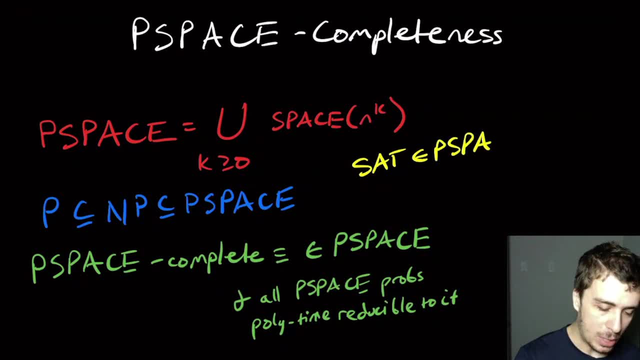 If I show that sat is in p space, then we are done, because any particular problem, other problem in np that you like, since sat is np-complete, we can just take that other np problem and reduce it to sat and we can run the polynomial space solution for sat. 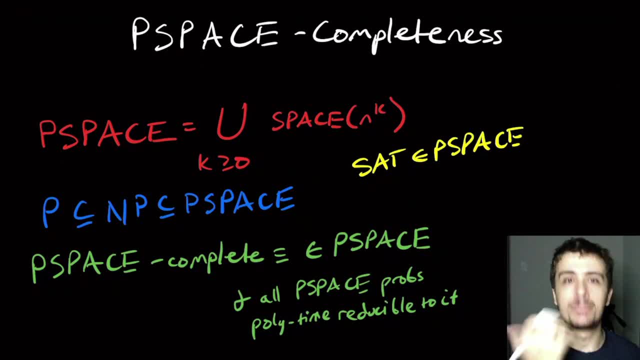 assuming there is one, and then we can get the answer for the other np problem, because the reduction only took polynomial time and hence only took polynomial space. So how do you prove this? Well, all that you do is you go through all possible assignments of variables in the formula. 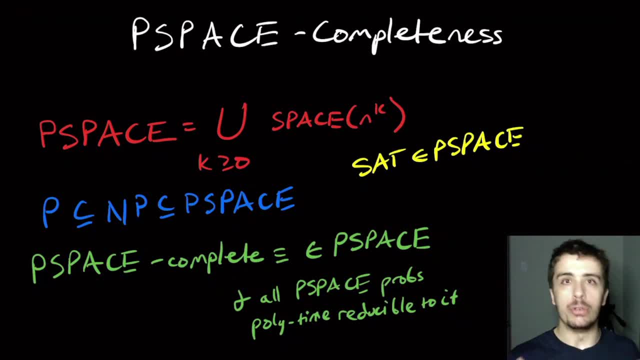 There are two to the n possibilities. What you would do if you were not smart is you would write down every single one of the assignments and then just evaluate the formula on each one of them. So what you would do is to write down one assignment, evaluate it If the formula ends up. 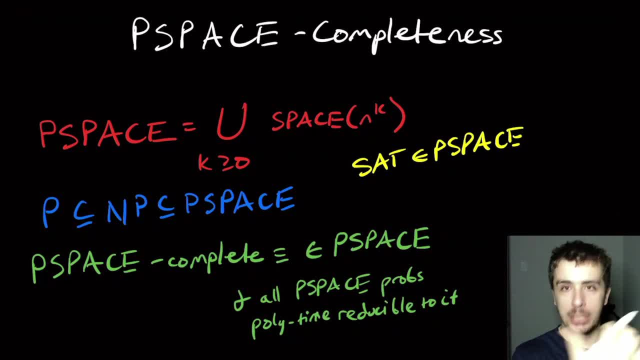 being true, then obviously we're done Otherwise: erase the assignment itself and then rewrite down the next assignment, And so therefore we will never use more than linear space in writing down the assignment, and maybe the evaluation of the formula takes an additional linear space as an. 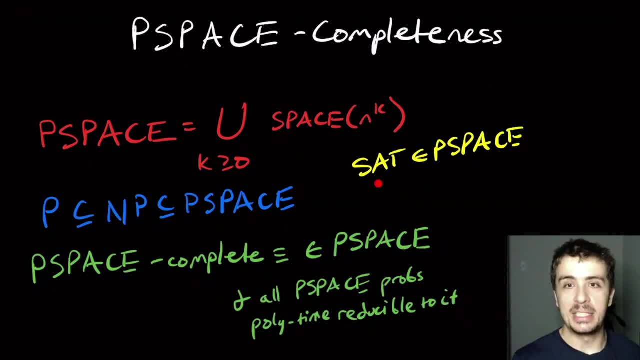 example, But in fact we can even show, based on that, that sat can be done in linear space, which is dang cool. But here that tells us all that we need. We just need to show this in polynomial space and that's all that we need. So np is a subset of p space And unfortunately we do not. 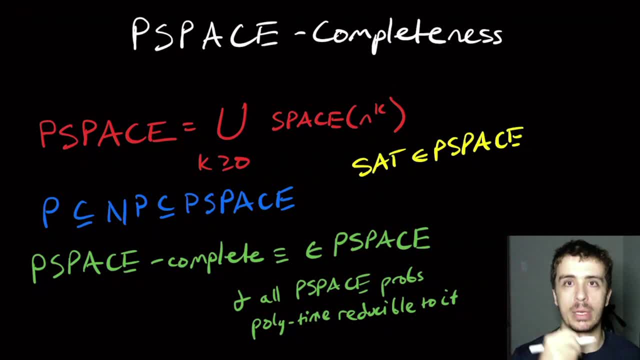 know whether these containments are strict as of the recording of this video. Knowing my luck, five seconds after I upload this video, it's going to be solved. But if you're watching this in the future and it's been solved, put it into the comments down below so that I can see and maybe 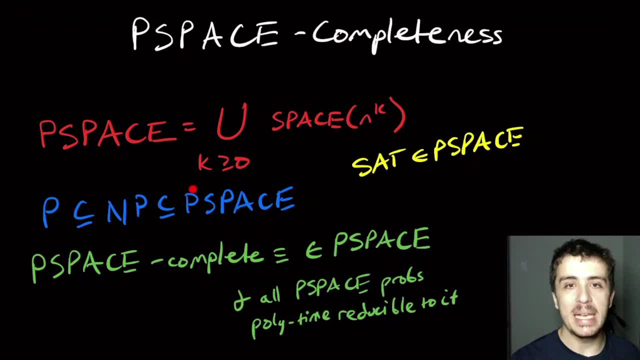 make an update. Anyway, we want to know whether p is strict from p space. In fact, all that we know, p can be equal to p space, although there's a whole lot of heuristic evidence to show that that's not true. 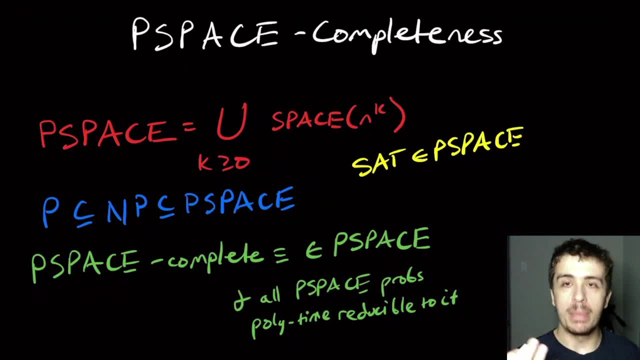 Anyway, we want to know what is the hardest problem that can be solved with a sufficiently small amount of space, polynomial space. Then we can actually invent a notion called p space- complete, kind of like np complete, but it's complete for p space. The idea being is that we 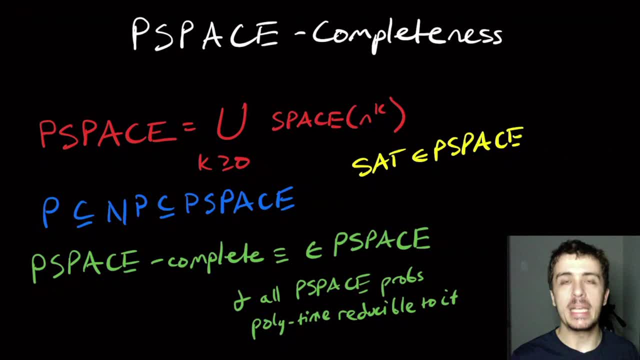 want to have a problem that is super, duper hard for p space and it's the hardest problem that can be solved in a polynomial amount of space. So the notion of complete in this sense is going to be that it's in p space If you're complete for. 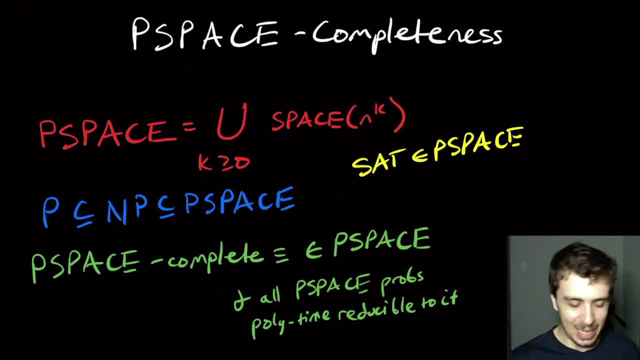 the complexity class. you better be in the class. But then we also have that every p space problem will poly time reduce to it? We don't want poly space here because that's the amount of space that we're allowed and that's not going to really help us all that much. 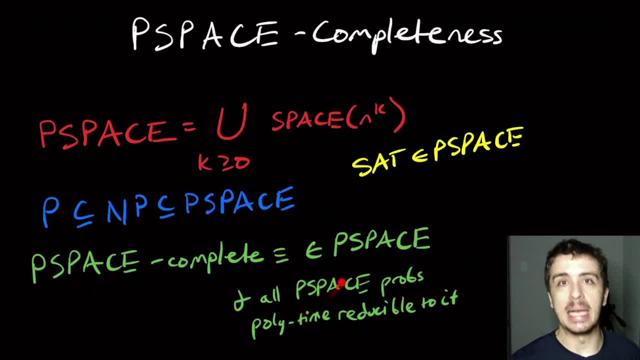 We want something that's strictly less, or we believe to be strictly less, than the amount of resources that we're allowed to use. So we're going to use polynomial time, And this notion right here is what is known as, as you might guess, p space hard. So to show that, 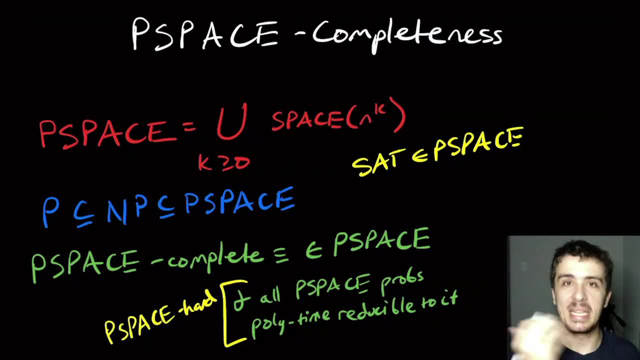 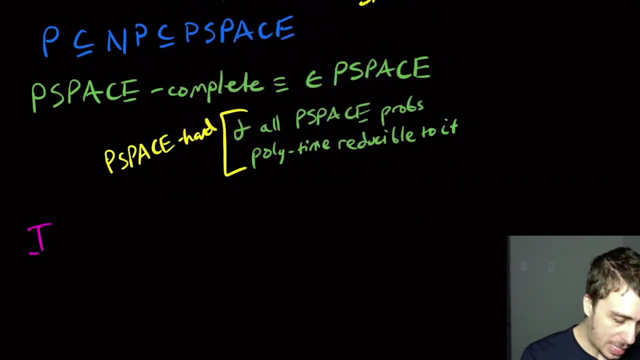 something is p space complete, all that you have to do is show that it's in p space and it is p space hard. So, for example, if we happen to show that sat is p space complete, we can show that np is equal to p space. So if sat is p space complete, then np equals p space. 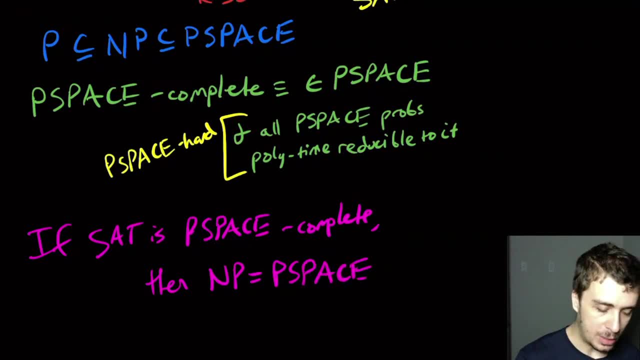 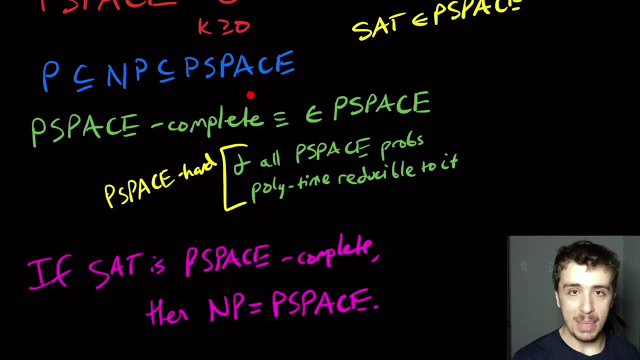 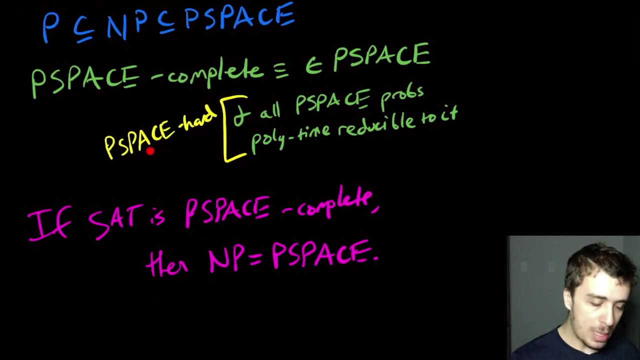 And this pretty much comes directly from the definitions here. So if it's p space complete, it already is in p space because it's in np And therefore, since it's a subset, therefore is in p space also. So if we know, 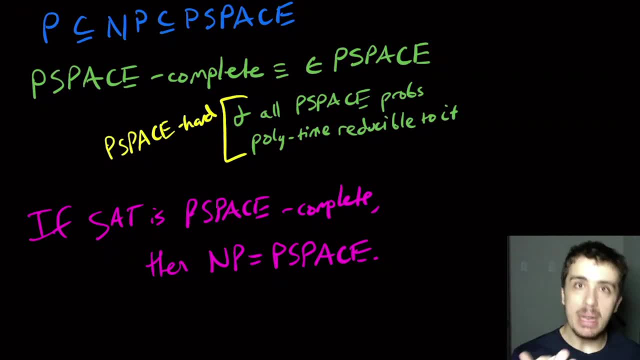 in advance that it's p space hard, then that means every p space problem can poly time reduce to sat, because we know that it's p space hard by assumption. And so therefore, take any problem in p space that you're concerned with and do the poly time reduction over to sat, And we know that it.